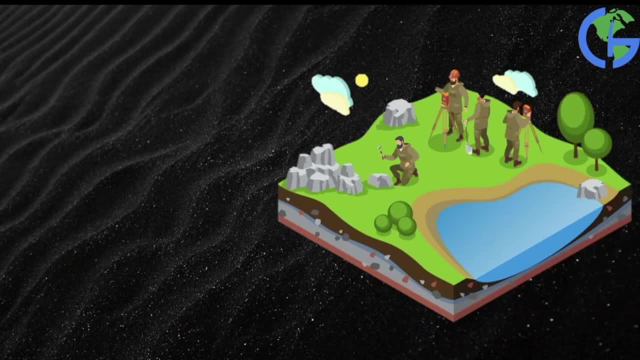 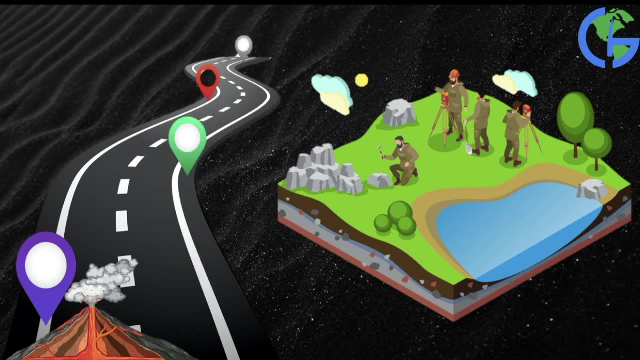 The need for a geological timescale came up when geologists wanted a framework to understand the sequence of events that occurred throughout the earth's history: Mega events like glaciation, volcanism, mass extinctions, intercalated with smaller events like sediment deposits. 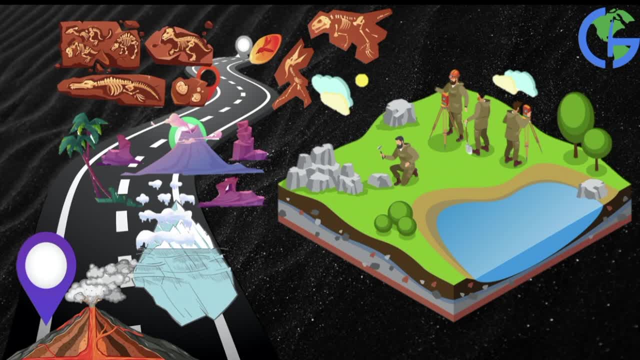 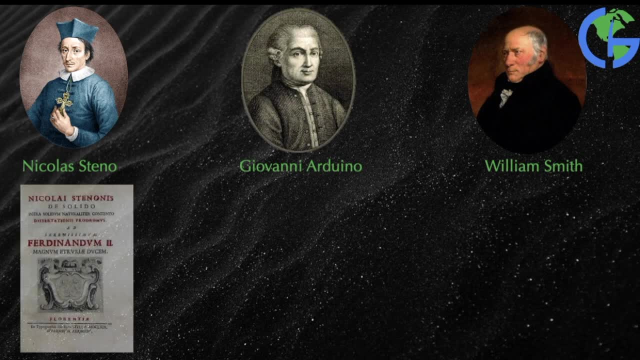 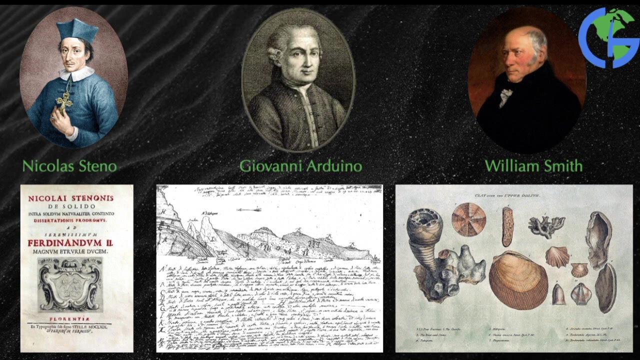 upliftment, erosion and others. Effort started back in the late 17th century to collect data about geological timescales. Nicholas Steno, Giovanni Audrino and William Smith were among the pioneers in developing the geological timescale. In the words of Arthur Holmes, 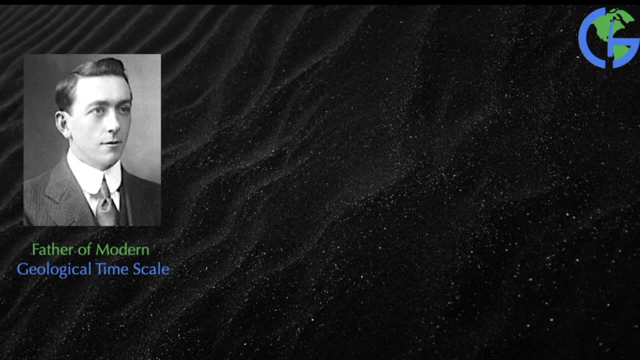 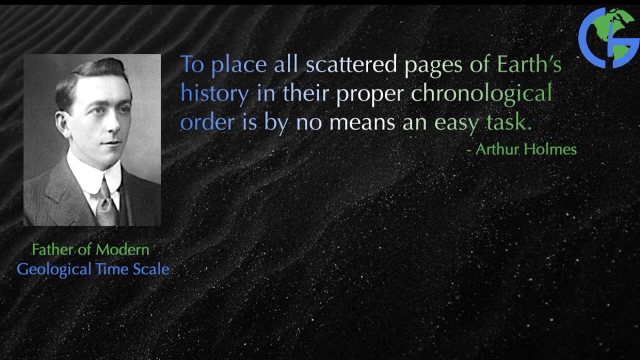 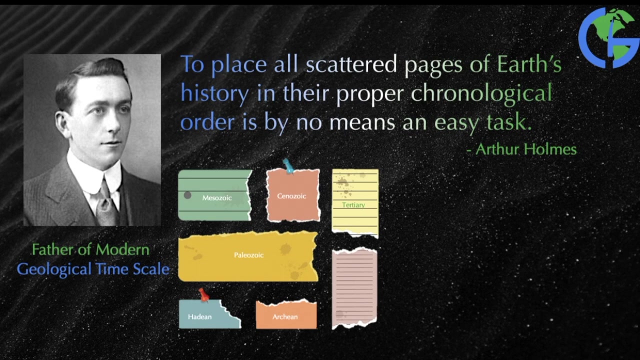 regarded as a father of geological timescale for his work in radiometric dating. to place all scattered pages of earth history in their proper chronological order is by no means an easy task. Organizing such scattered and torn pages requires a very detailed and accurate timescale. 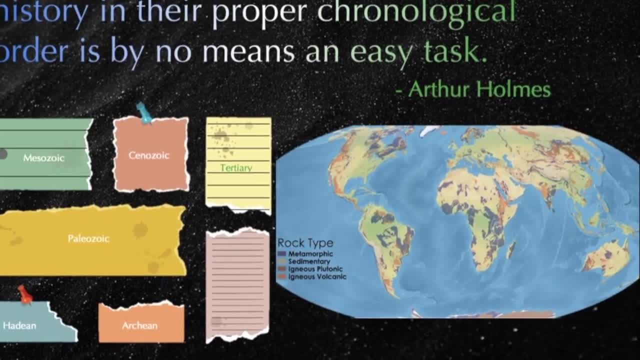 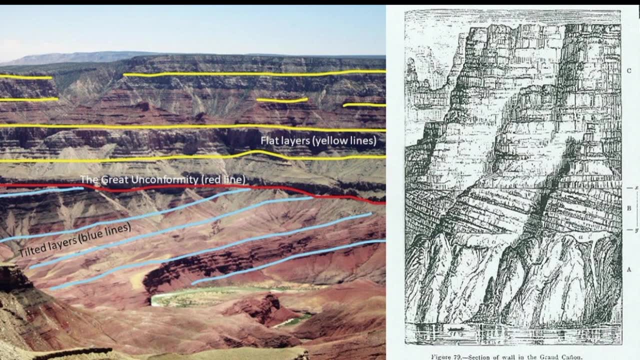 Describing any duration of geological time requires a fairly good preservation of continuous rock records formed in that duration, which can provide us clues as to what happened at that point in time. As a geologist, you must have the necessary tools and knowledge to literally unearth the truth. Adding to complexity, it is the fact that there is no single locality. 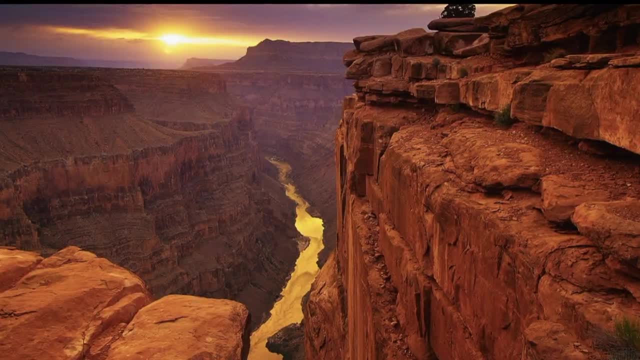 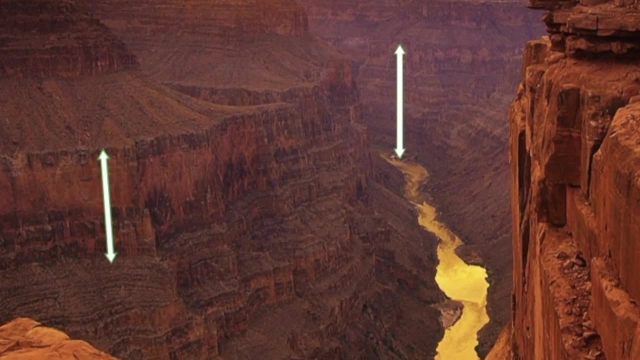 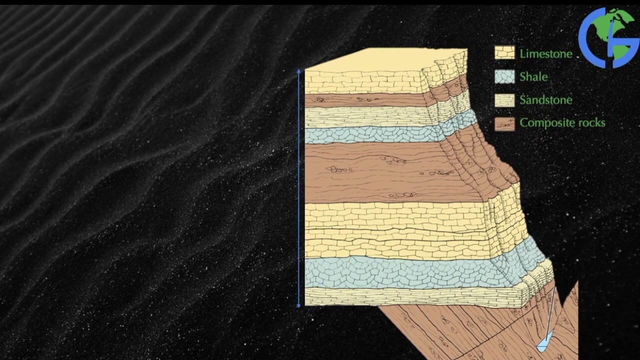 that exists on earth where a complete sequence of rock formed continuously throughout the geological time is available. The great canyon carved out by the Colorado River in USA preserves a great deal of history. Developing a framework requires a lot of cooperation at international level and, in this regard, the first international geological congress took place in 1878, France. 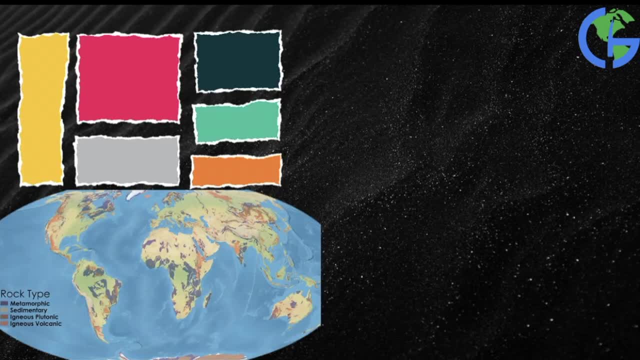 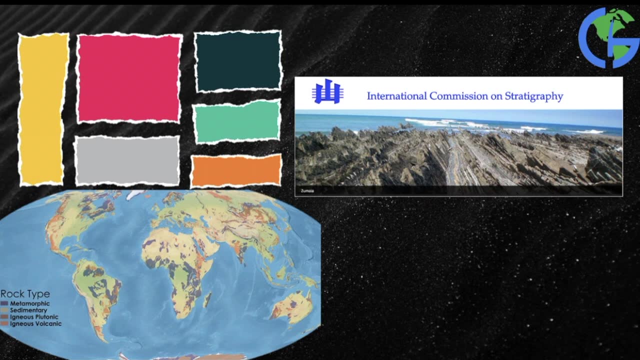 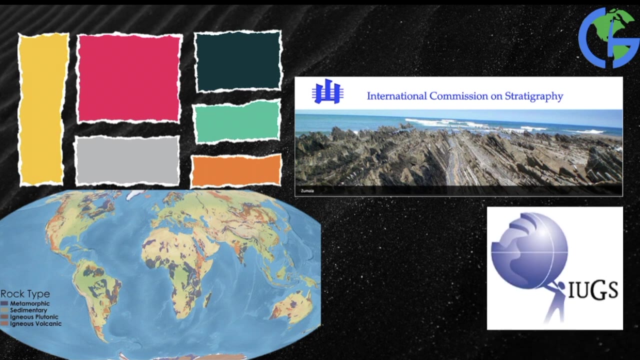 Where large amount of data started pouring in from various locations, there was a need of standardization. Since 1974, international commission on geography, ICS, a subgroup within International Union of Geological Sciences, IUGS, has attempted to establish a standardized global geological timescale. 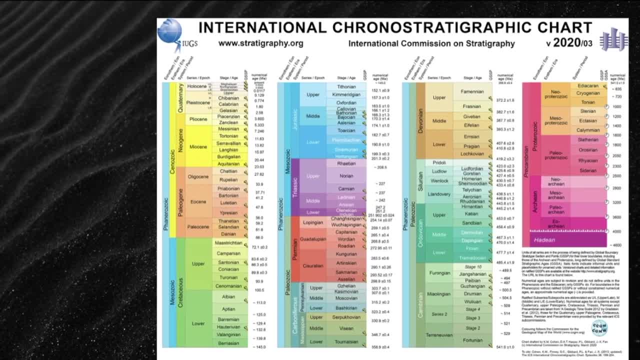 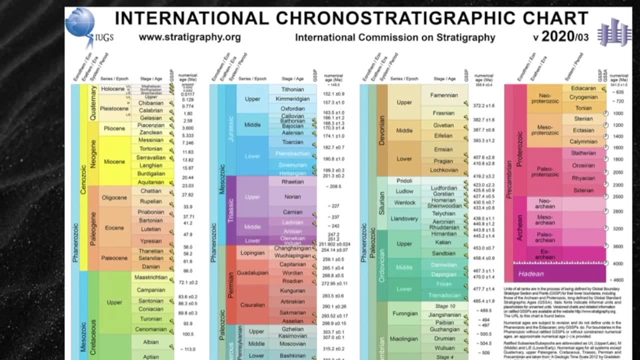 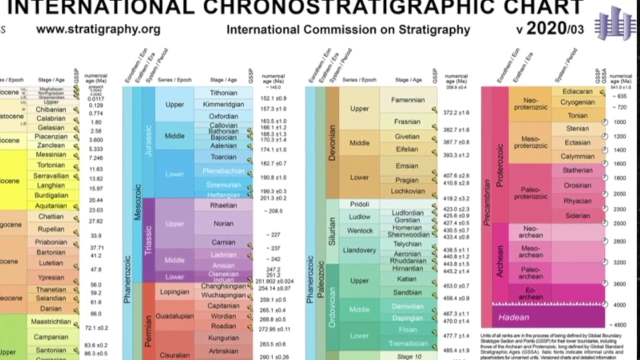 With the advances in geological science, new methods for finding age have come along, and old methods have also improved, thereby increasing our resolution of time. Our accuracy has also reached a very high degree of precision, but there are still some blurred regions. Geological timescale is a systematic chronological arrangement of events occurring in space and time throughout. 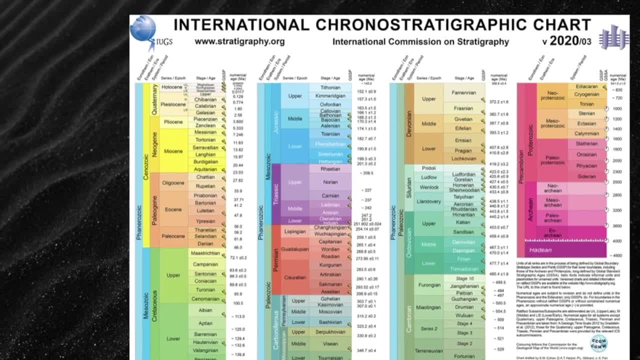 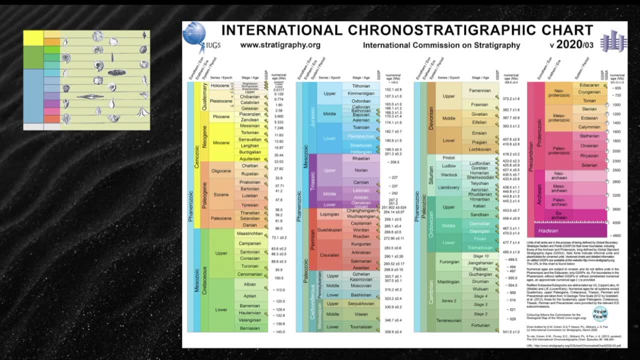 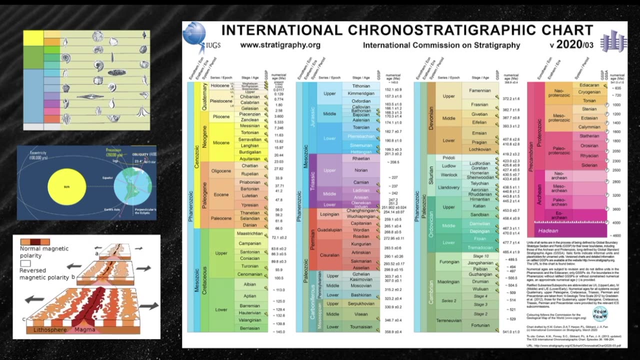 the earth's history. Techniques that are used to achieve this gigantic task includes radioactive dating of elements, paleontological zonations from fossil records, Milankovitch cyclicity, magnetic reversals astronomically tuned in cycles in linear time, and few more. 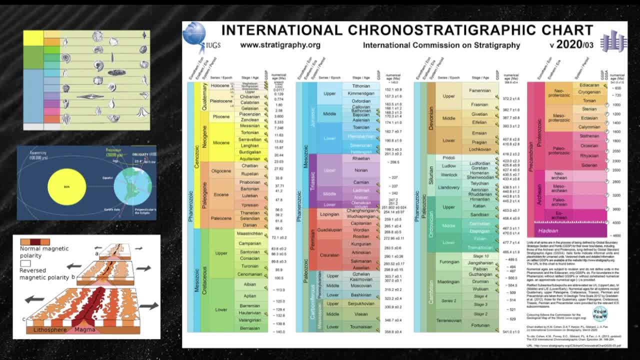 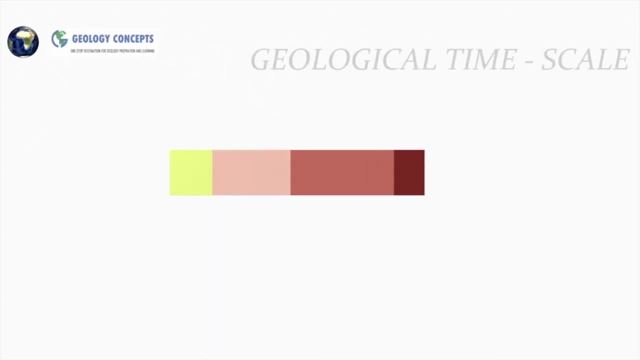 Each of these techniques use a proxy that is related to time and can give us the idea of the earth's history. Now, as we know the beginnings of geological timescale, let's look into the major divisions in it. Primary divisions of geological timescale is called eons. Earth's geological history is: 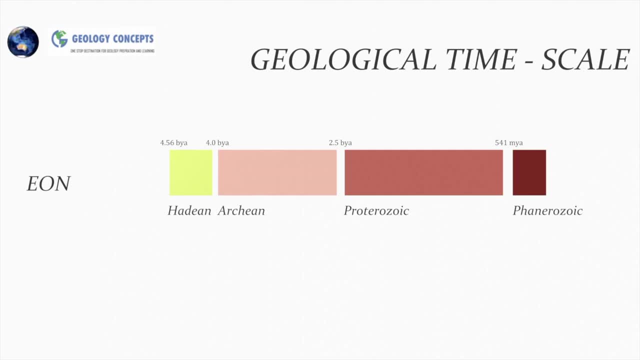 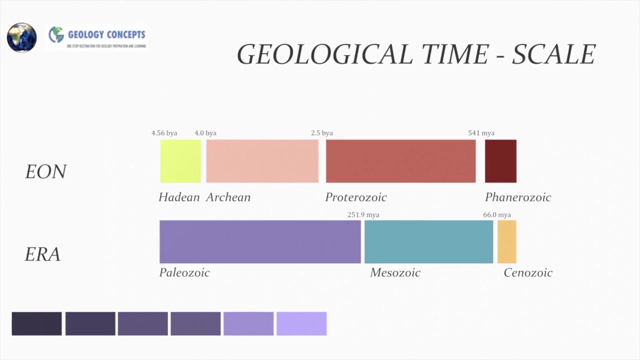 divided into four eons, namely Hadean, Archean, Proterozoic and Phanerozoic, which we will understand in subsequent videos. Eons are further divided into eras. It must be told that each of these boundaries between those divisions represent some characteristic change at that point in the 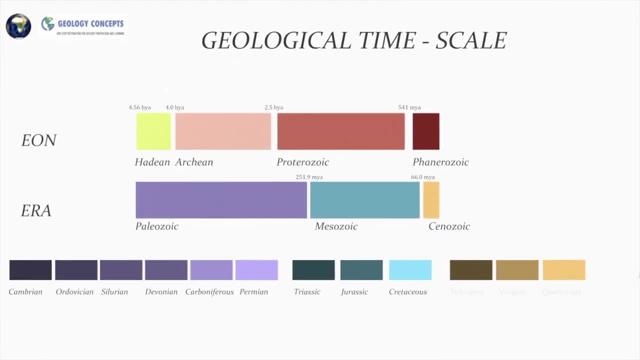 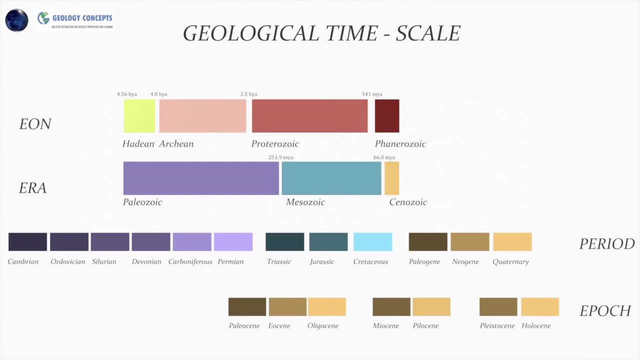 earth's history Era, as we go further, is divided into periods. Periods is divided into epochs and epochs into ages. Relation between these time divisions and rock units lies at the heart of geology. Such correlation will disclose the sequence of events that occurred in time and space. 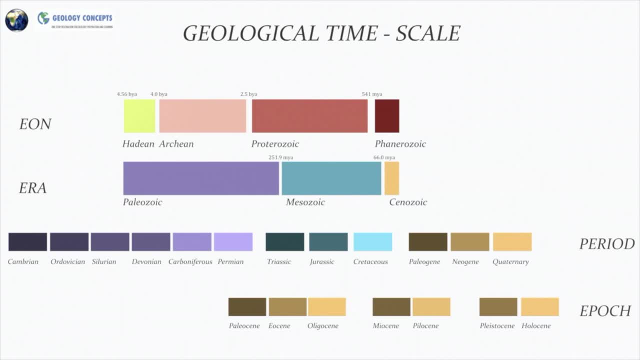 Rock units that refer to specific time in geological timescale are called chronostratigraphic units Corresponding to these divisions in geological timescale. their chronostratigraphic terms are used to refer the rock layers that belong to the earth's geological timescale. 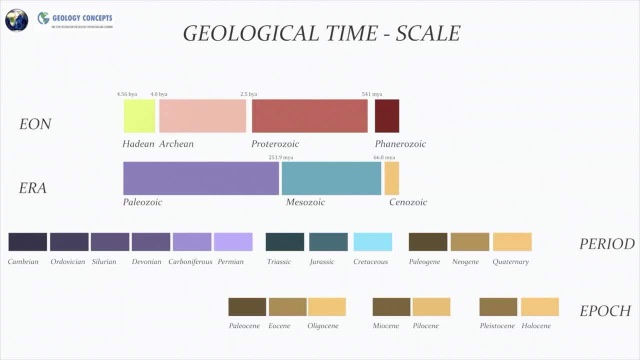 Earth's geological time is also linked to the geological time point. in geological timescale, Those are called geological time points. On one hand, you now see the geological time levels that belong to these stretches of geological time in the earth's history. Rock unit corresponding to eon is called eondem. 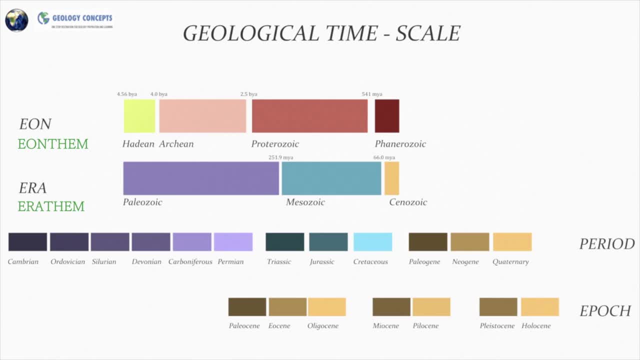 Eradem corresponds to era- unit of geological timescale System, to periods, Series, to epoch, and stages correspond to the age unit of geological timescale division. Now, since we have a fairly good idea of geological timescale origin and divisions, we can start with. 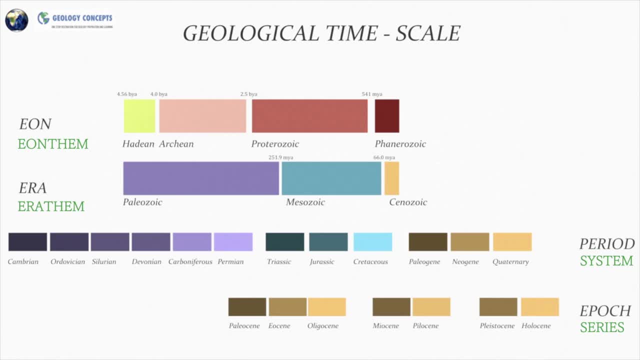 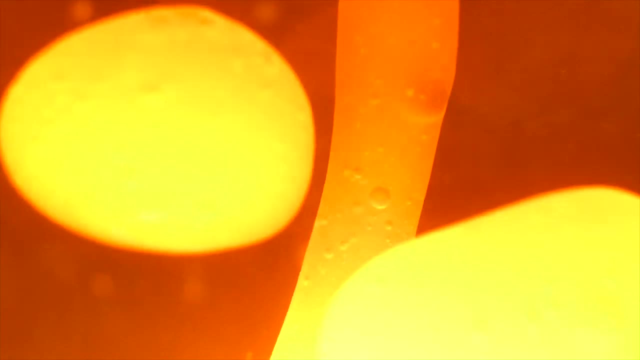 understanding each division in detail. So in next episode I will explore each division and try to understand what earth was like during those times and what were the major events that took place and gave earth the shape as we see it now. I am excited to take off this journey of 4.5 billion years with